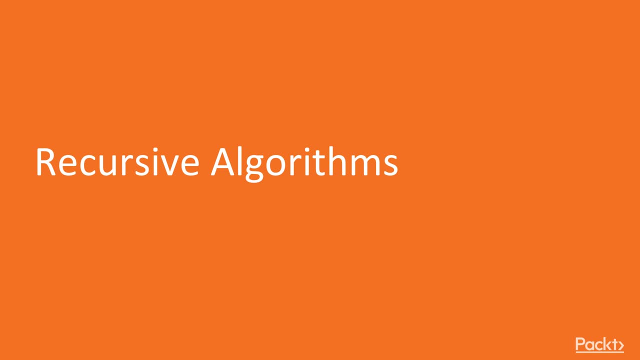 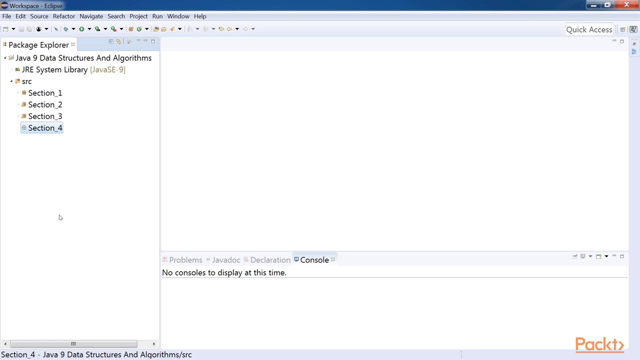 Now we move on to the first video of this section that deals with recursive algorithms. In this video we are going to look at examples regarding recursive algorithms. Recursive algorithms are a different way of thinking about solving a problem. For example, say, our problem is to write a program that, given a positive integer n. 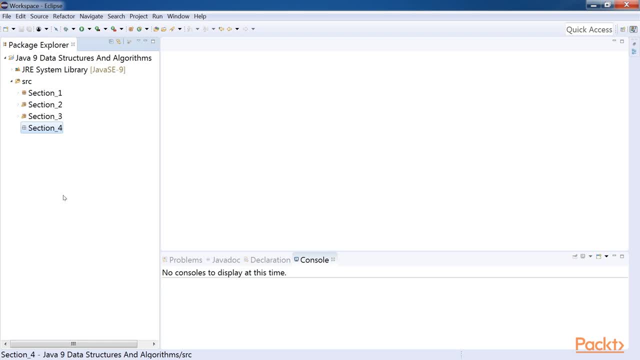 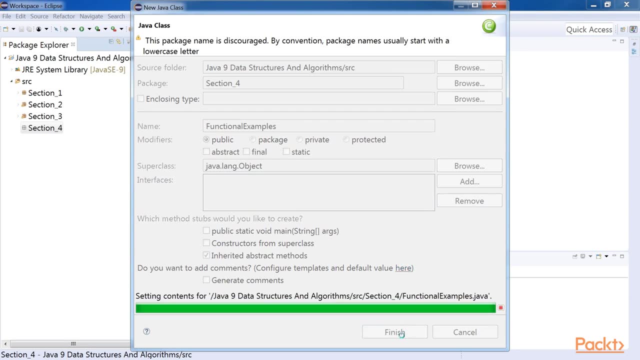 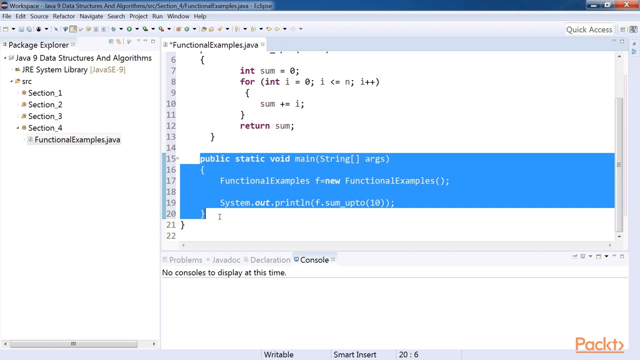 returns the sum of numbers from 0 to n, The known imperative way of writing. it is simple. Let's create a class named Functional Examples. This is a sum-up-to method. Add the main method that calls sum-up-to method. We calculate the sum up to 10.. 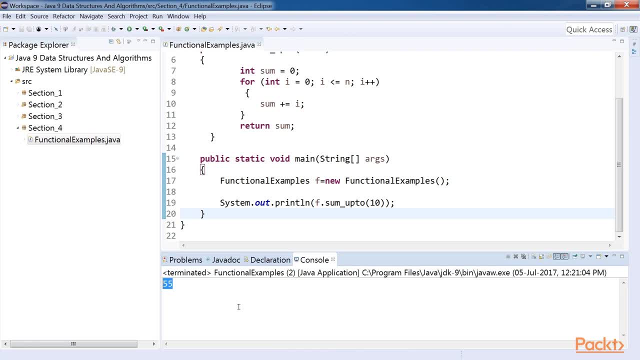 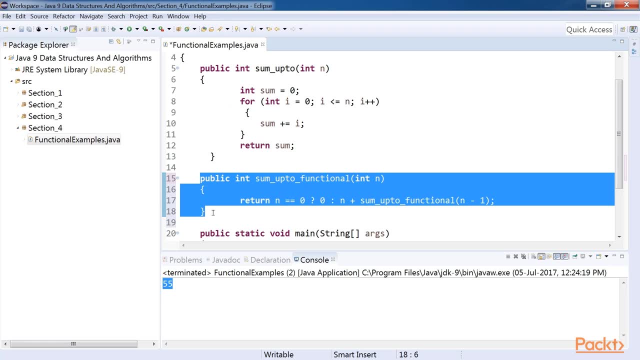 So when we run it, we get 55, from 1 to 10.. Let's see the functional version of the problem. That's it, Just a one-liner. This is probably nothing new to Java programmers, as they do understand recursive functions. 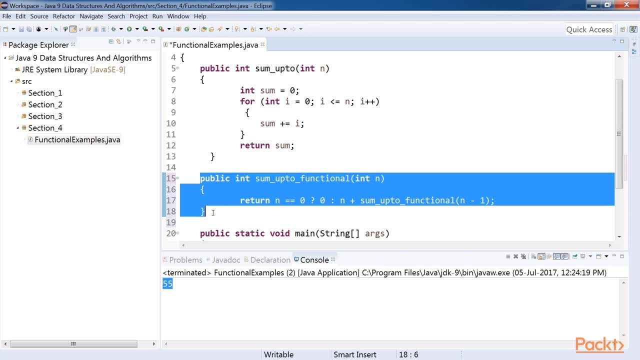 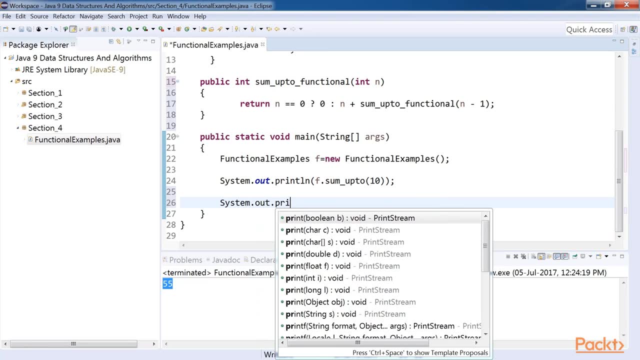 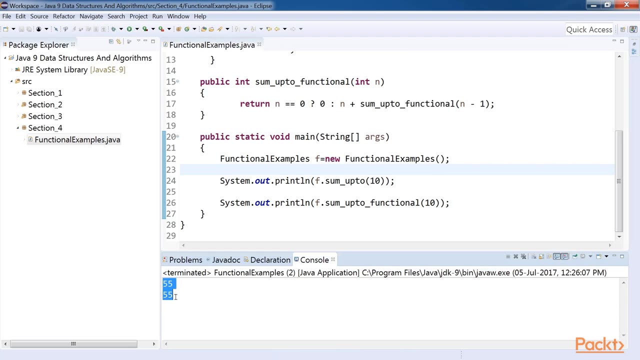 However, an imperative programmer would use recursion only when nothing else worked. But this is a different way of thinking. Now let's call this sum-up-to-functional method from the main method. We've passed same inputs in both the codes. Let's check the output. 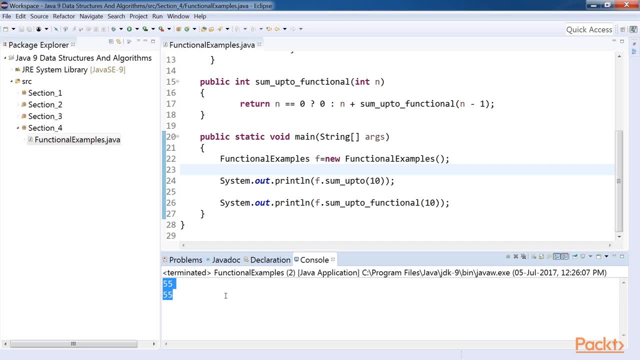 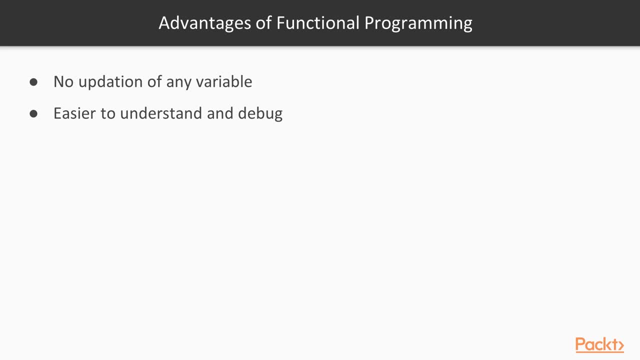 You can see that both give the same output. In the imperative version we are updating the variable called sum for each value of the loop variable i. However, in the functional version we are not updating any variable. What do we achieve by that? 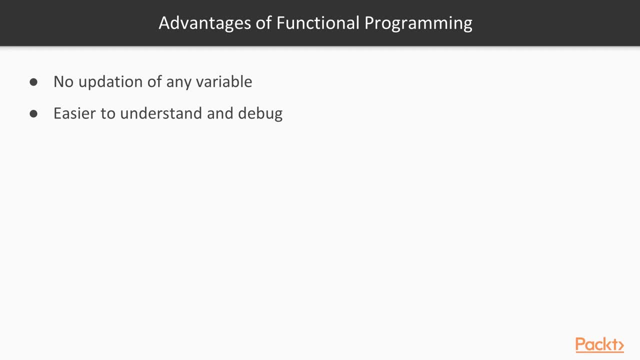 When a variable is updated multiple times in a program, it is hard to understand or debug it, because you need to keep track of the latest value. When this does not happen- When this does not happen, When this does not happen- it is far easier to understand what is happening. 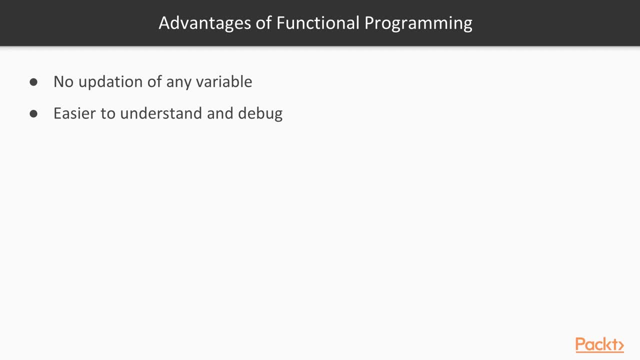 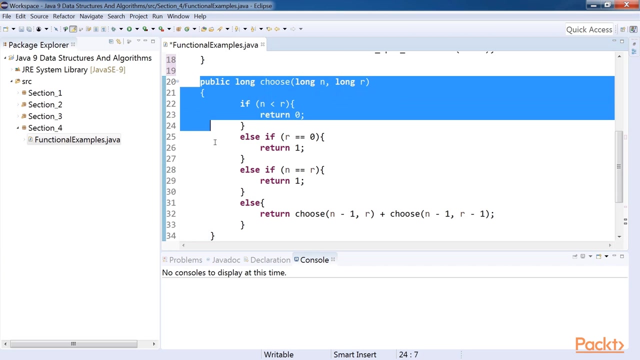 In fact, it makes it simpler in such a way that we can even prove the correctness of the program completely formally, which is rather hard to do for imperative programs where variables change values. Let's check out another example. This one is about choosing r objects from n objects, where the order does not matter. 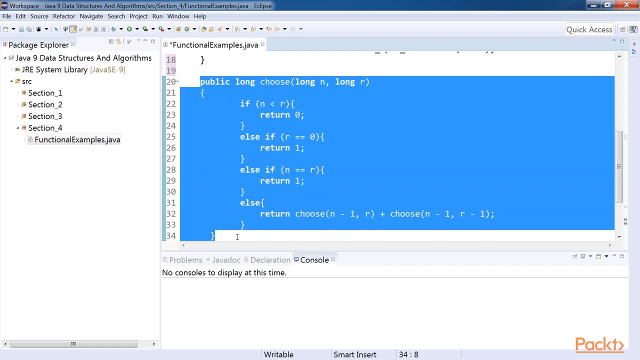 Let's have a set A of a finite amount of objects. Let the number of objects in the set A be the number of objects in the set A. Let the number of objects in the set B be the number of objects in the set B.